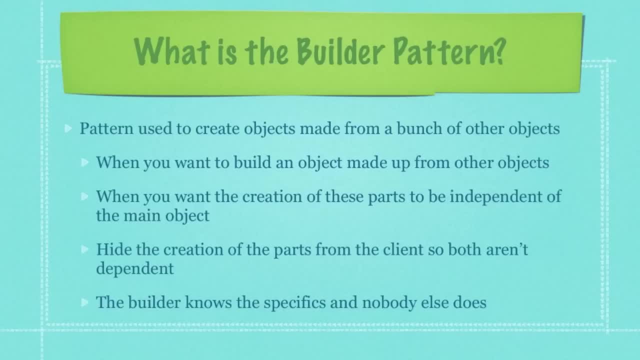 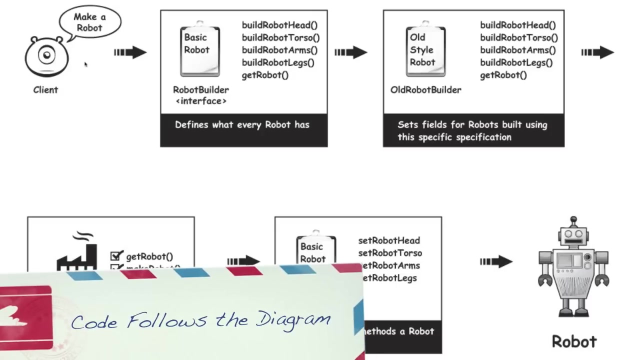 specifics and every other class involved knows nothing about what's going on. in regards to the specifics of the final object, you're going to create Sounds way more complicated than it is, and now you're going to see how simple it is. Here is the builder pattern. Basically, I'm using my old alien here and in this situation he is going. 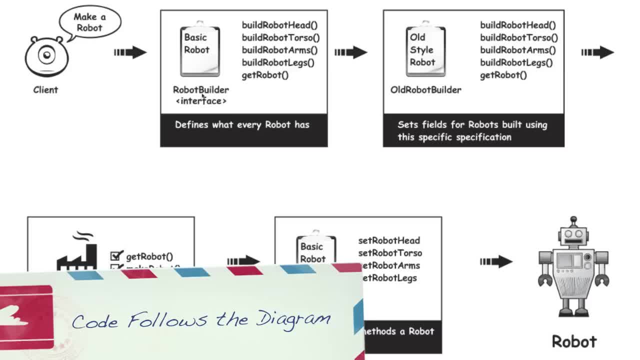 to request a robot to be built for him. Here is the interface, which we're going to call robot builder, and it's going to find what every robot has, which means a method that builds a robot- head, torso, arms and legs- as well as receives the robot. Then, of course, you're going to implement this interface. 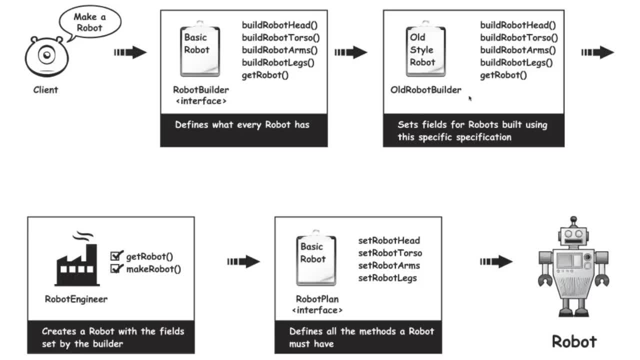 over here with the old robot builder is what I'm going to call it- and then you just need to implement all those methods, And what this guy does is it's going to start all the specifics for making a very specific robot type and here is the final robot, and it's going to have a whole bunch of fields This guy up here is going. 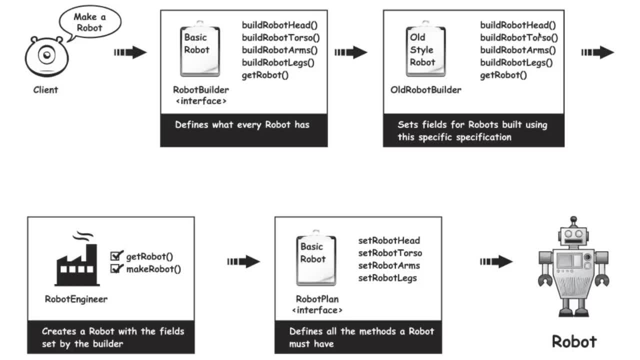 to set the values for those fields whenever build robot heads called and Build robot torso and so forth and so on. and of course Git-robot is going to return this Robot to whoever calls it, mainly this little alien over here. Then were going to have the robot engineer, or what is often called the. 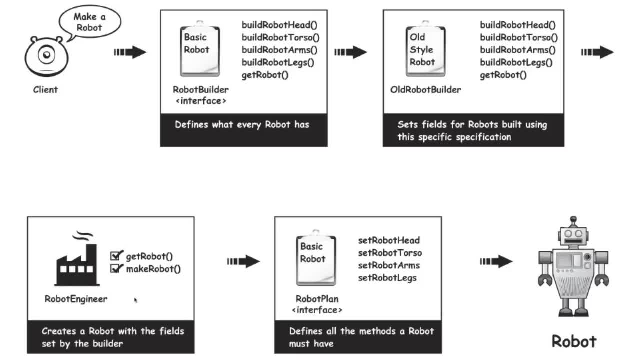 Director, and what it does is it creates a robotbor, Create a robot for it, Give it exact number. Same thing to do with the robot we ran into The CTR robot. editing creates a robot with the field set by the builder, this guy up here, And then, finally, we have our 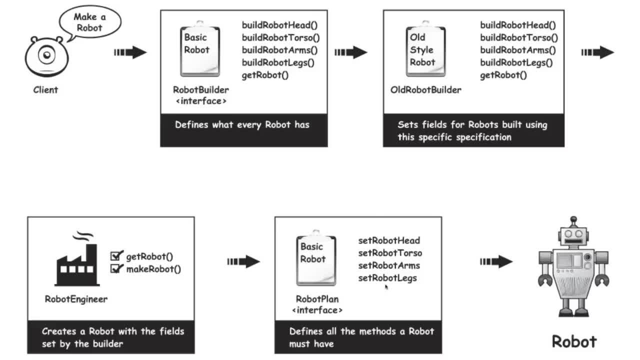 interface which is going to have all our set methods to set all the values for our robot and then the final robot itself. So now we're going to go from this basic little diagram here to build all of the code. So on with the code. So here we are, inside of Eclipse, and the first 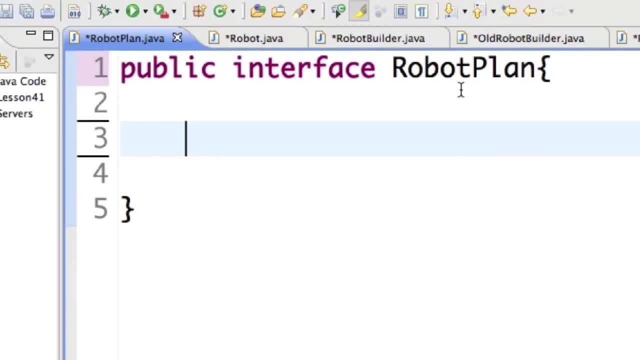 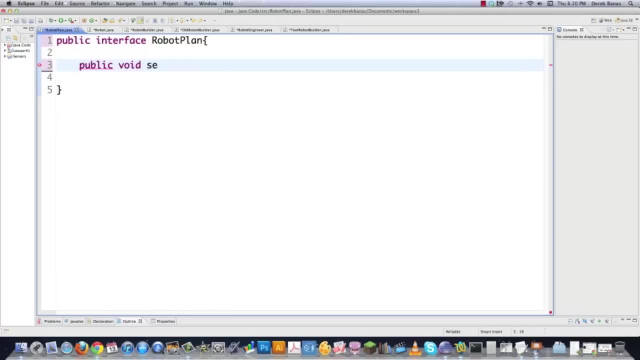 thing we're going to do is come to robot plan, which is going to be the interface for creating all of our robots. This is real simple. we're just going to, just like always, define all the methods that need to be set up. So we're going to say that we want our robot to have a head, and it's going to 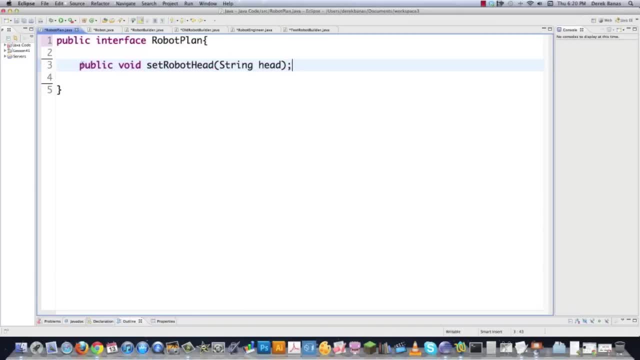 be past a string and we're just going to call that head. So real, simple. And then we're also going to define our torso, our arms and our legs, And then this is going to be past torso, arms and legs. So 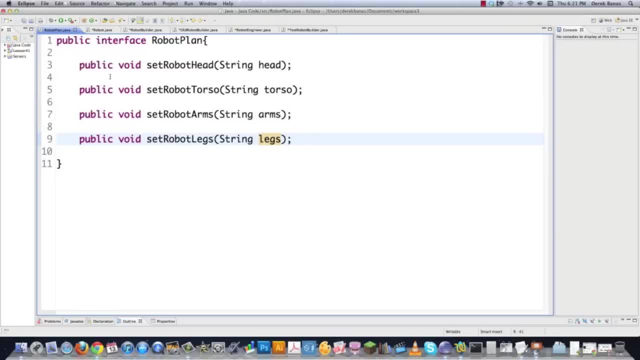 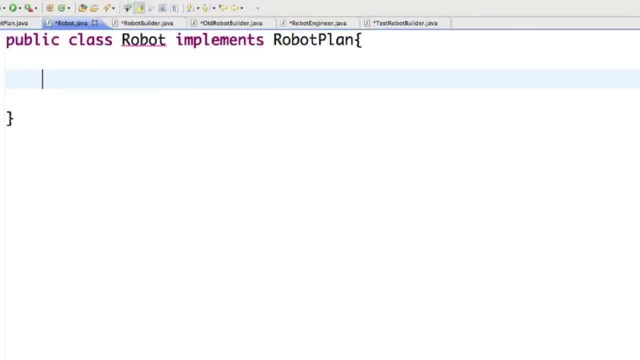 here you're going to define all the qualities that you want all of your robots to have And then, after that, you're going to go to robotjava and you're going to implement the robot plan which you just created. And if we come up here, we're going to just put our mouse over robot and it's going to say add: 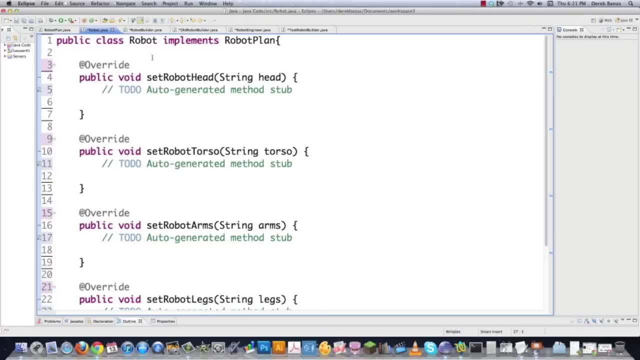 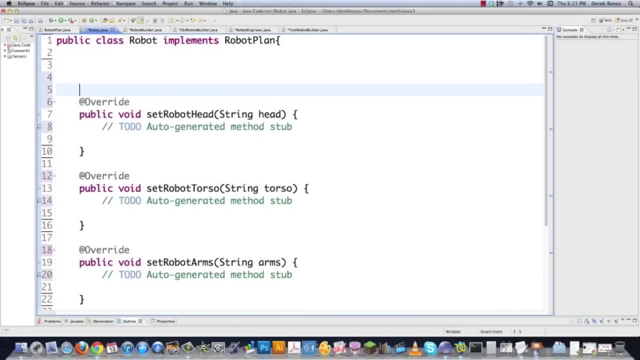 unimplemented methods. We're going to do that and there we go, And this is going to act as the concrete robot class, based off of the interface that we just saw right there. So what are we going to need to do? Well, we're going to need to actually create these fields for ourselves. So they're all. 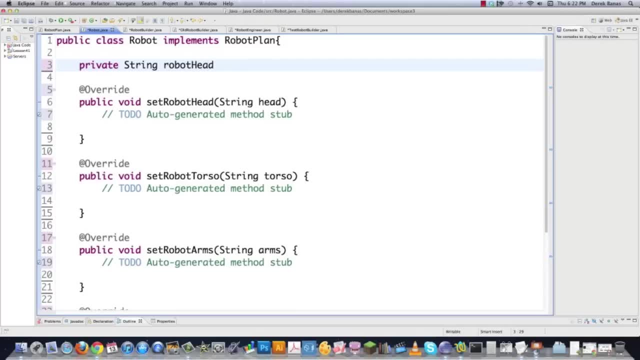 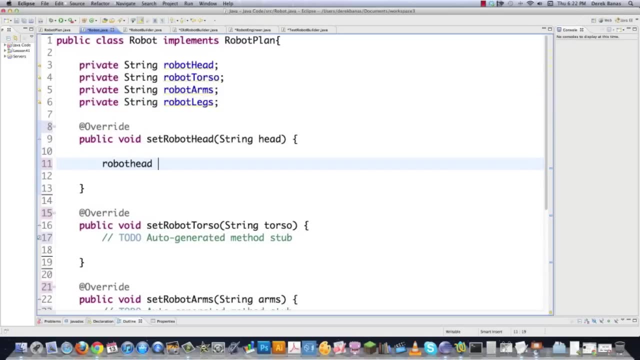 going to be private, of course- String robot head, robot torso, arms and legs, And then what we need to do is just come in here and go: robot head is equal to robot head, And then we're going to go to whatever the value of head is robot torso And make sure that we put this as upper case, of course. 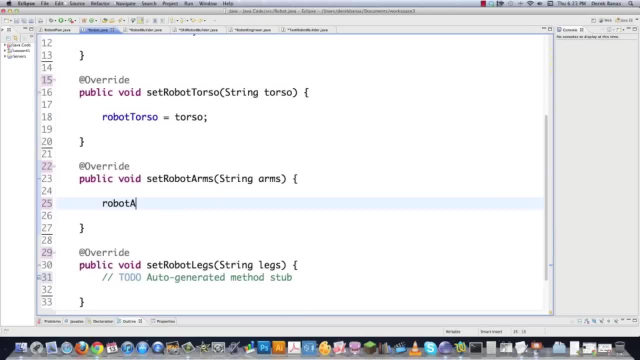 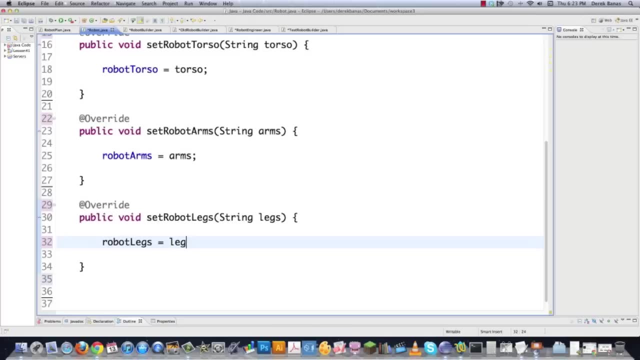 is equal to whatever torso was when it was sent over, Robot arms is equal to whatever the value of arms was, And robot legs is going to be whatever the value of legs was. And there you go, Got that all set up. Now. the only other thing we're going to want to do here is put some get methods inside. 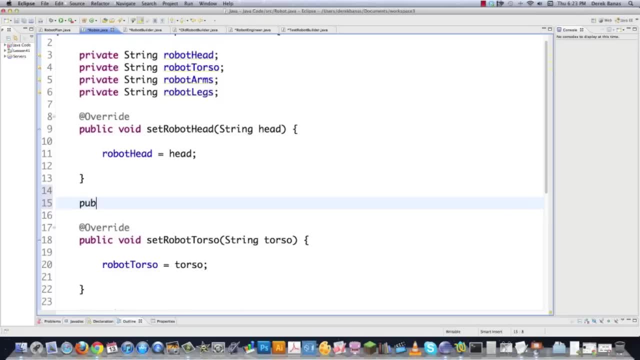 Most of the time, whenever you have set methods, you're also going to have get methods, So we're going to go public string And all of the code that is here is an unimplemented set And what you're is available underneath the video. you should get it if you really want to learn this stuff. it's. 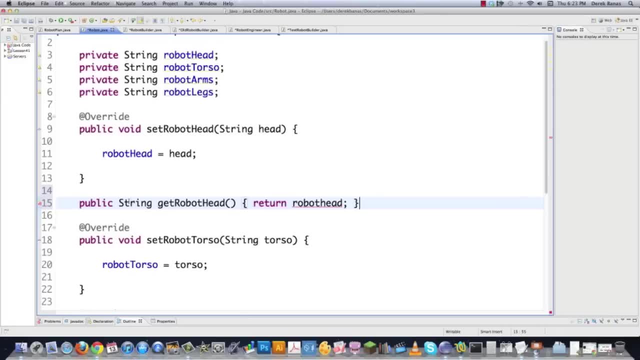 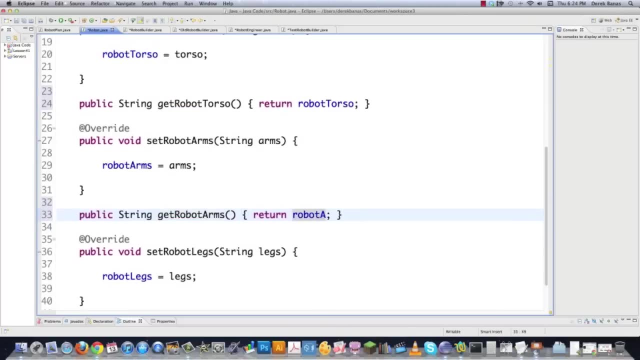 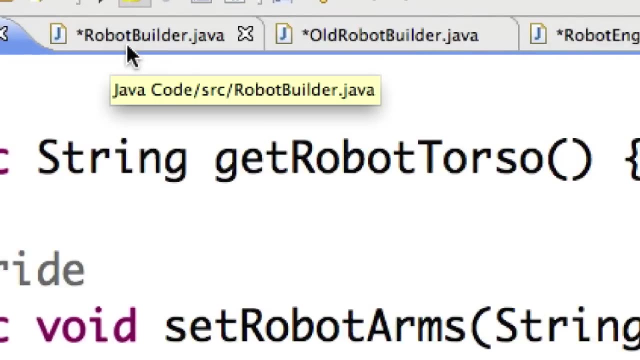 free. why not? okay, return robot head, real simple. and then we're just gonna also do the get methods for the torso, torso arms and arms and legs, and there you go. that is all we're going to do with robotjava. so now we need to come in here to robotbuilderjava, which is going to be the 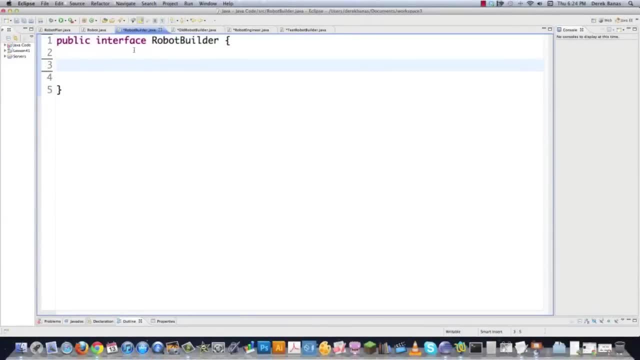 interface for building all of the different types of robots we want to use. so what sort of things are we going to want this guy to do? public void? well, we're going to want to build our robot head. of course, using interfaces just makes everything so simple. don't have these long classes, everything. 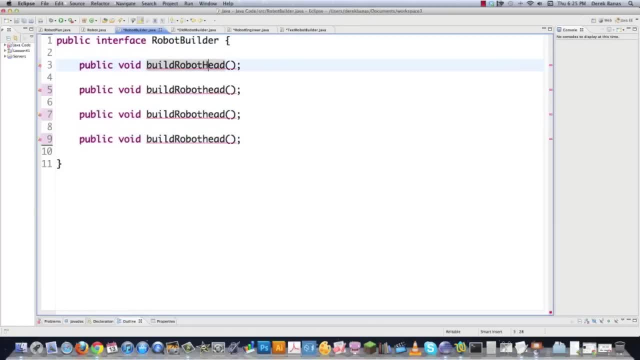 is going to be real easy to implement and you don't have to think that much. i'm going to make that uppercase and this is going to be torso, arms, legs and there you go. that's all it took to create the basic interface for robotbuilderjava. now we're going to create old robot builder and this: 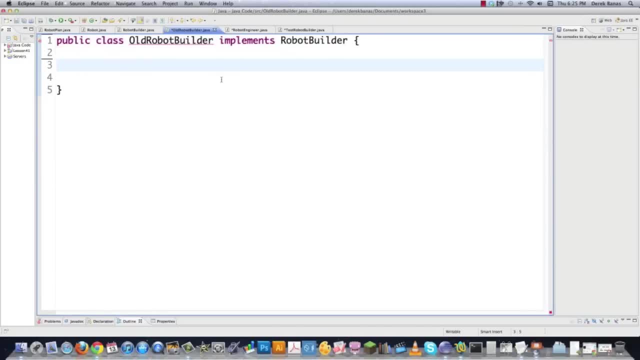 is where you're going to see all the changes, because this is going to be the basic interface, going to be the concrete builder class that's going to assemble all the parts for the finished robot object. so we're going to have to go private robot because this is going to be building a robot. 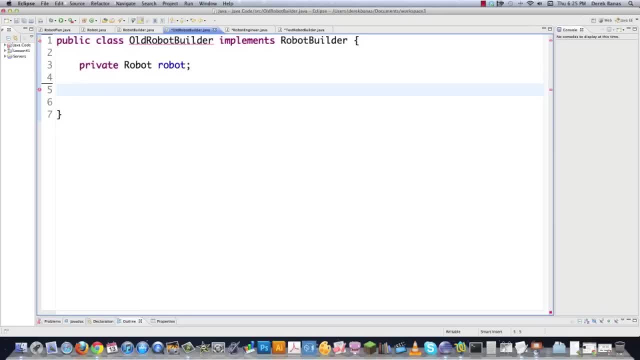 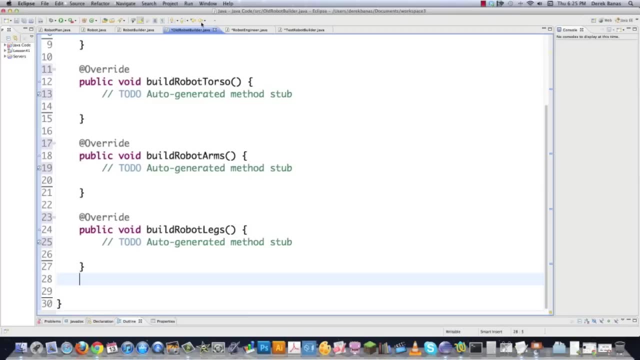 so we're going to need access to an actual robot object, and then there's no use typing all that out, because we can just put our mouse over this guy, of course, and go add unimplemented methods and there you go, got all our stuff automatically thrown inside of there. and now, since we have 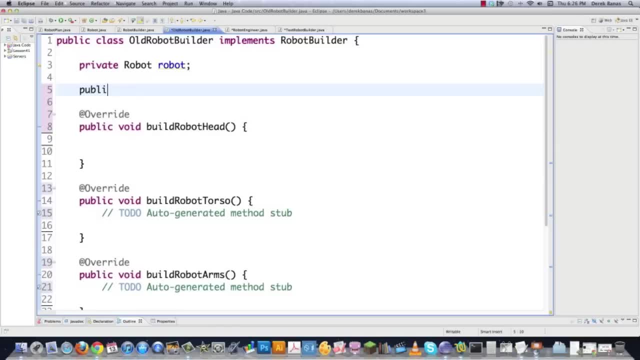 robot defined up inside of here in a compositional type of way where the field is actually an object a la the other strategy pattern, sort of kind of we're going to come in here and define this robot, which is a reference to this robot up here right there, is equal to new robot. so now we have that. 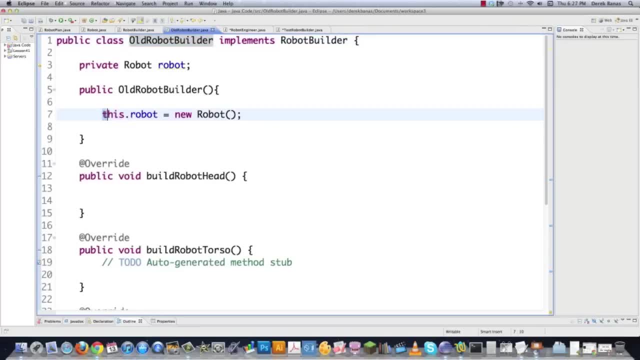 guy all set up, and this is the constructor, of course. so we know that this robot is going to be created whenever this guy is called. so that's good. and then what we need to do is just go robot dot, set robot head and since this is an old robot, let's say his head is made out of tin, just to do. 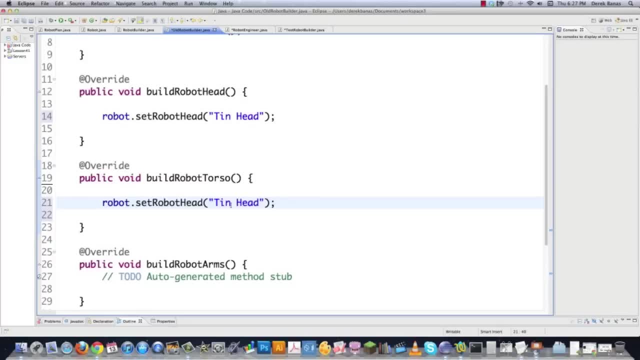 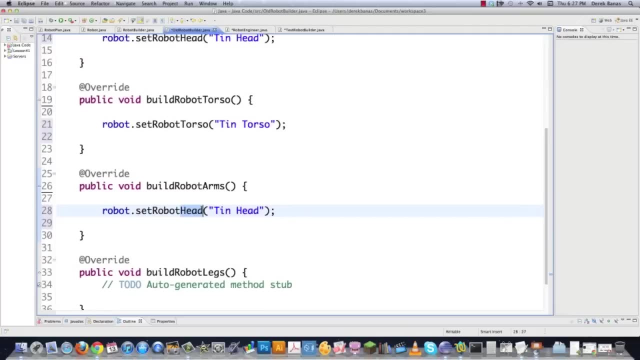 something, and you see, all i'm doing is calling all the methods that were defined inside of the robot class. so set robot torso and this is going to be tin torso arms. what would be an old-school type of arm for this guy to have. how about a blowtorch? blowtorch arms. and then we come down. 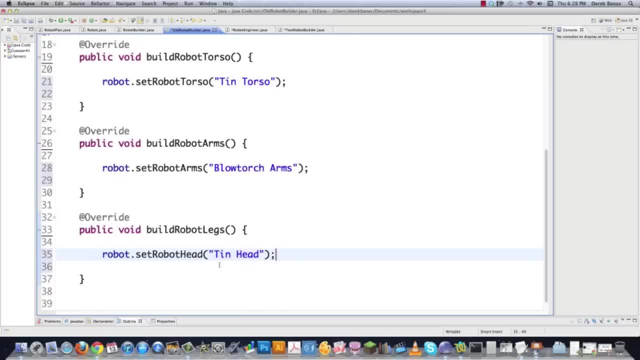 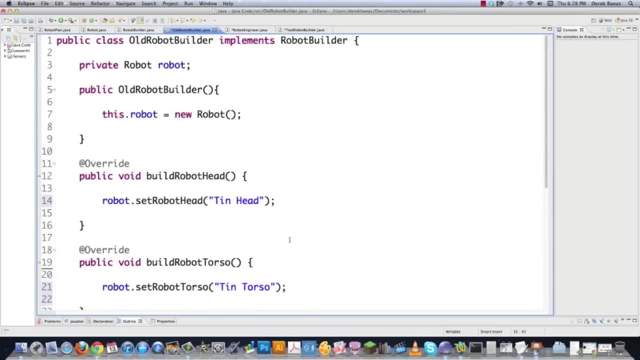 to robot legs and what would be an old-school type of robot leg? how about roller skates? so this is a roller skating robot with blowtorch arms made out of tin. and there you go, there's the old robot builderjava. and every single time you want to. 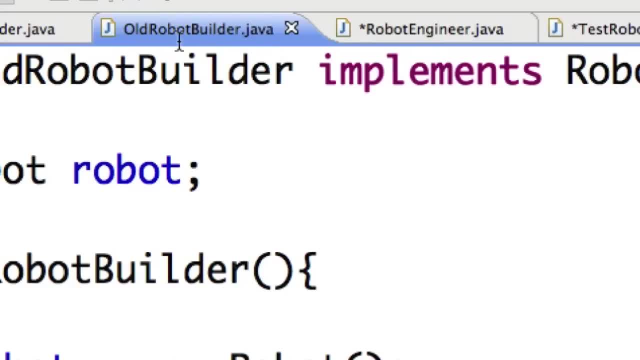 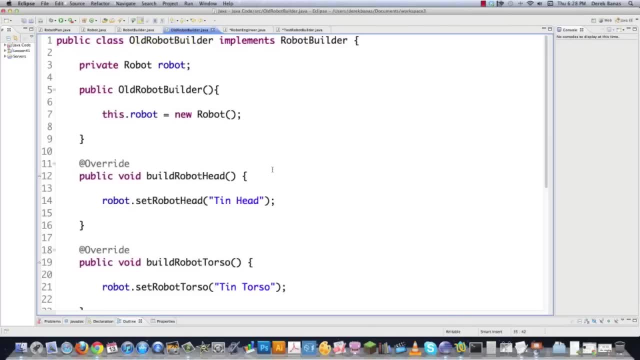 define a new type of robot. you're just going to create a new builder object that's based off of the main robot builder interface which we just created, and everything is just going to work. so now we come to the robot engineer, which is what i call it. a lot of people call it a director, but 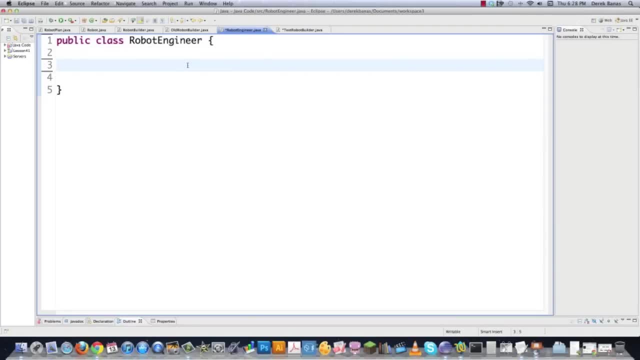 i just have always called it an engineer, so that's what i call it. and what this guy is going to do is create a robot using the builder interface that is defined right here, with old robot builder in this situation. so what are we going to do? we're going to go private. 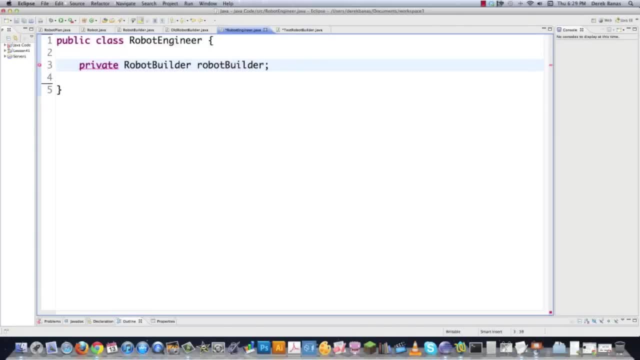 robot builder. robot builder is going to be its name, and then we're going to call robot engineer, which is going to be the constructor, and it's going to be passed a robot builder specific object, which is going to be our old style robot type here, and then, once again, we're just going to 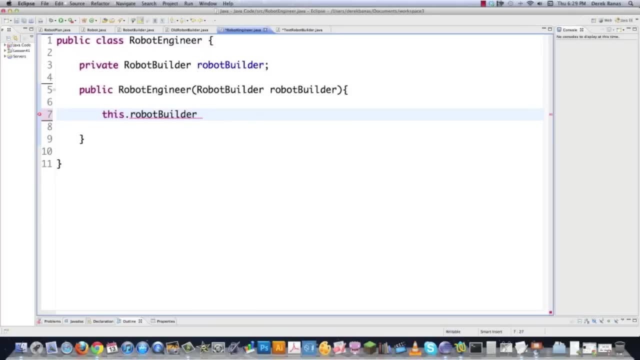 go this robot builder. you can think of it as kind of like a factory type, right like that. so we know we have a robot builder or we have a factory for building robots and this guy back here has robots inside of it. so you can think of it this way that this guy defines this factory type. don't call it a. 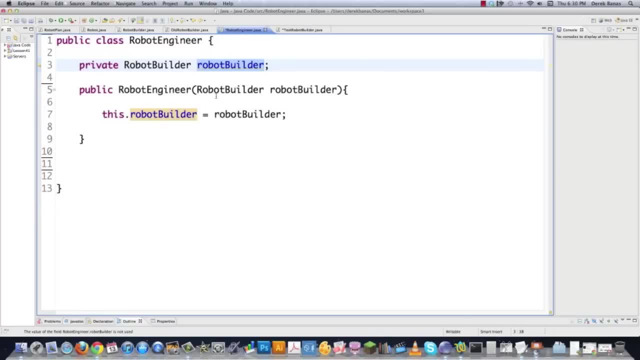 factory. but you know, if it makes you understand this better, you can think of it that way. so we're defining the robot builder factory area and over here we're defining the robot itself inside of old robot builder. so that's how we're able to backtrack and actually create these guys. so what? 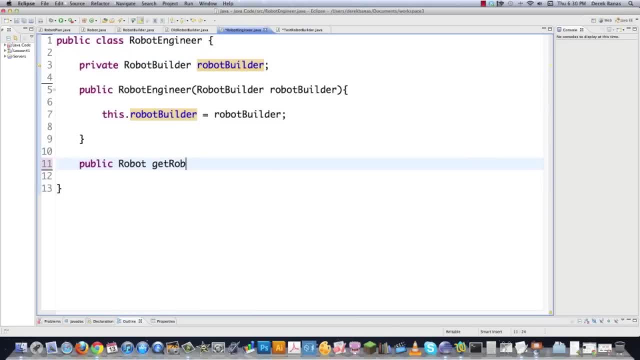 So what do we need to do with this? Well, we're going to have to provide the option for get robot, so that they'll be able to get the robot that is created inside of here by the engineer, And to do that, we're just going to go return this robot builder: get robot. 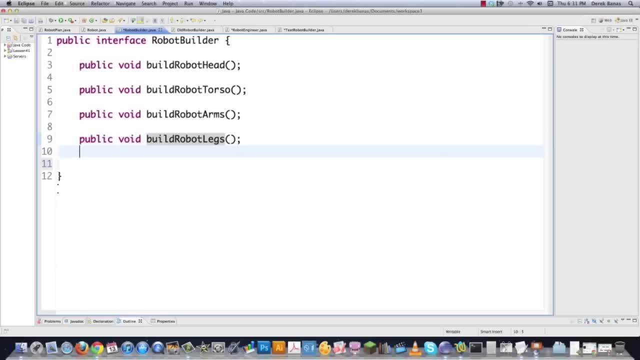 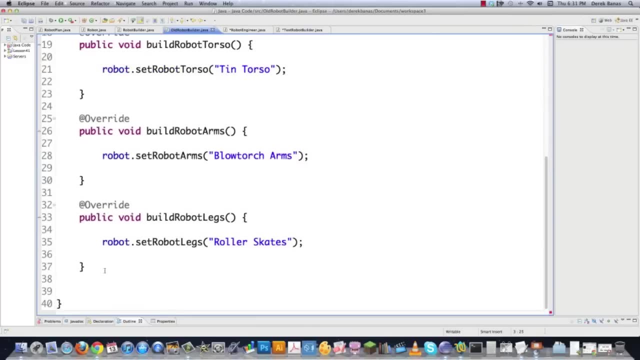 And to do that we're going to have to go over here to robot builder dot Java and just go public robot get robot so that it will be able to return that and then bounce over to this guy right here which is the old robot builder dot Java which implements the robot. 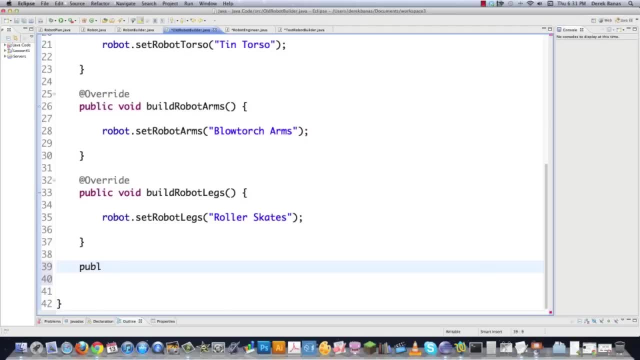 builder itself And then, of course, come in here and implement: get robot, There you go, And what's it going to return? It's going to return this robot which this builder knows how to create. So pretty simple: bounce back over in a robot engineer. 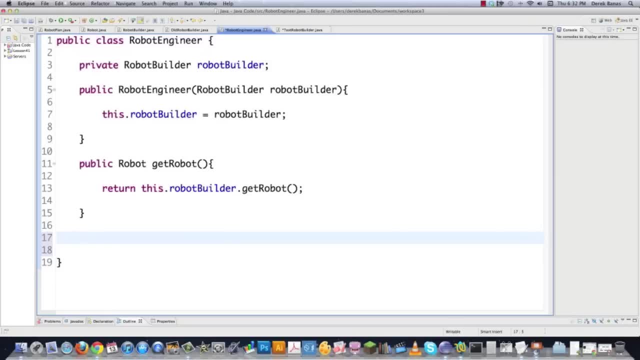 And then what the robot engineer is going to do is execute the methods that are going to be specific to the robot builder. So to do that, we're just going to go public: Avoid Robot like that. And then we're going to say this robot builder. 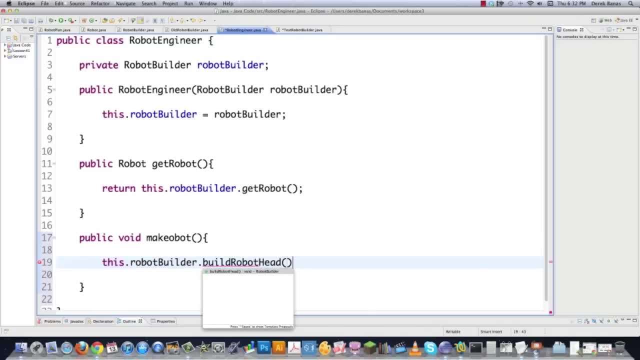 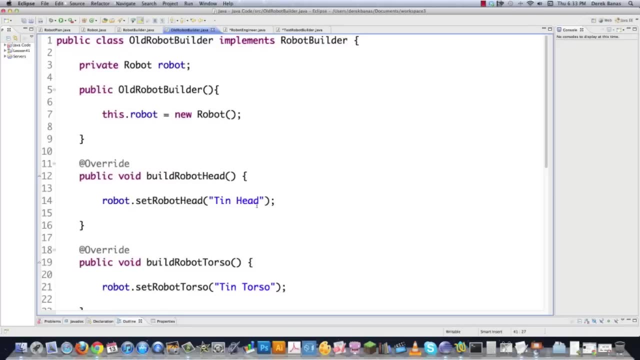 We want to call the build robot head method, like that, which, of course, is right here- Build robot head. And what's it going to do? It's going to set the value to 10 head for head inside of robot, which is back over here. 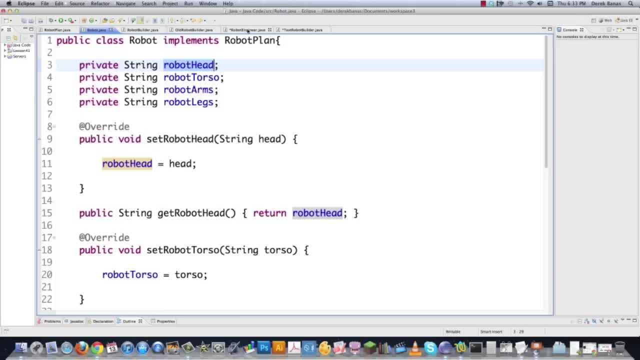 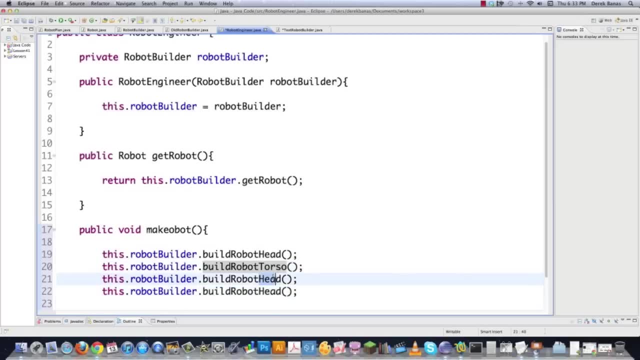 And you can see right there there's robot head. So that's exactly what it's doing, So bounce back over here. So what do we need to do now? We just need to set all the other values for the torso And the arms and the legs. 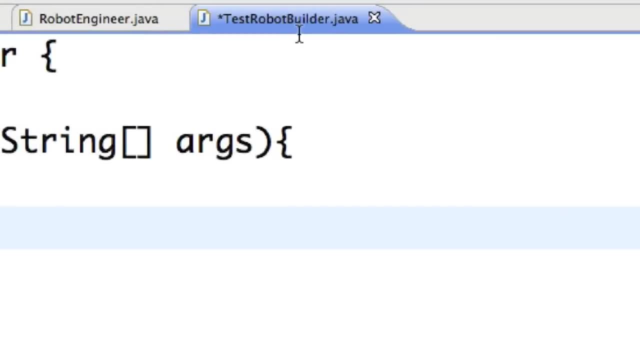 And that's it. So I'll save that. And then we're going to go into test robot builder and we're going to check to make sure we did all this right. So what are we going to need to do if we want to build ourselves a robot? 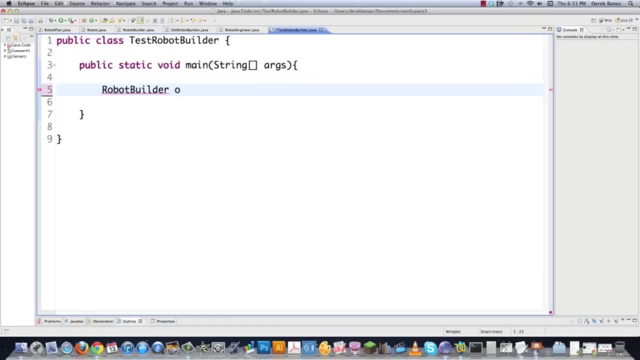 Well, we're going to need to get ourselves a robot builder object, obviously, and I'm just going to call it old style robot, And then it's going to be of type old robot builder, So you could think of it as if you're saying: OK, I want to get myself a robot builder. to. 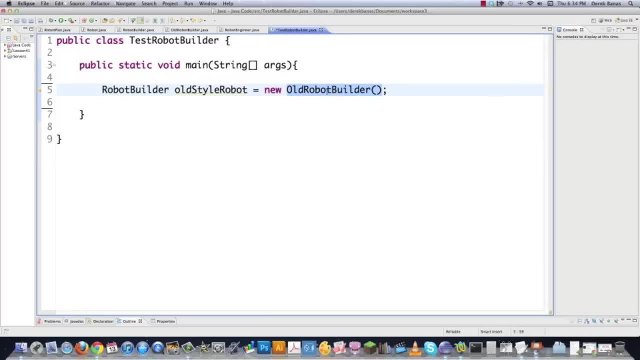 build me a robot, And this is the class blueprint that I want you to use to create that robot- And then what we're going to need to do is pass the old robot builder specification to the engineer. So if we want to pass something to the engineer, well, we're going to have to actually create. 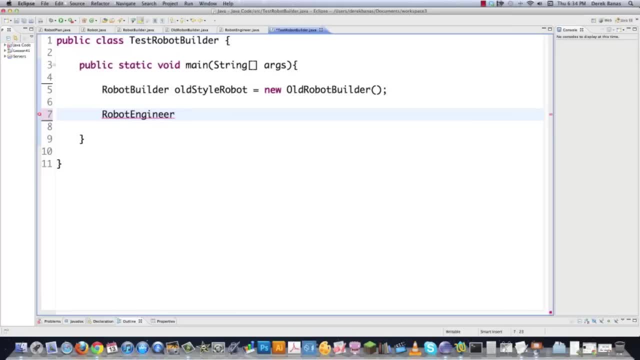 the engineer And I need to spell engineer right. And there we are. So we defined that we want to get ourselves a robot builder. We wanted to use the blueprint defined in old robot builder And then we need to get ourselves an engineer to build it. 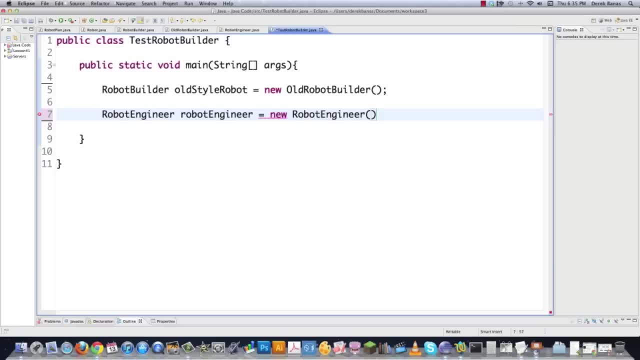 And this is going to be equal to new robot engineer And we need to pass over the specs that we created right here, or the blueprint for what type of robot to create. And there we are, We did that. And then we need to tell the engineer to make the robot using the specifications of the 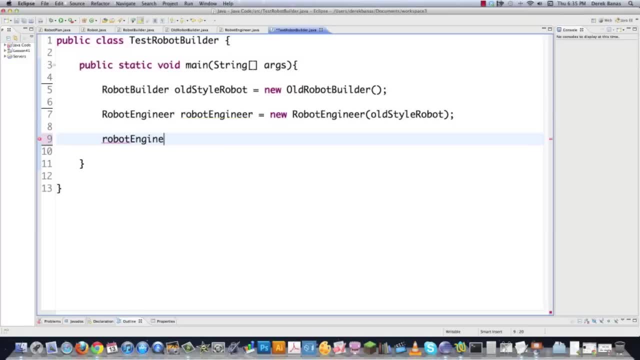 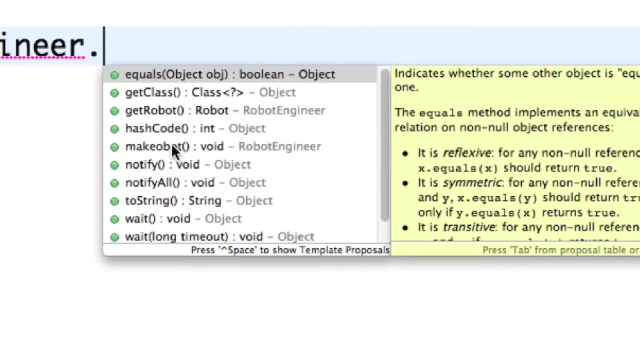 old robot builder class. So we're going to go, robot engineer, put a dot there, And then what's it going to say as our options? Well, one of our options is make a robot. Well, that's definitely not going to be the right thing. 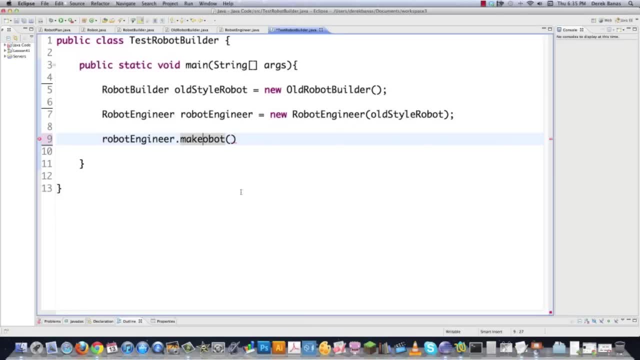 We'll click on it. What did that tell us? That told us that we need to change that to robot, Make robot. And then jump over here into robot engineer and change this to make robot. There we are. Nice way to catch our little errors we've made there. 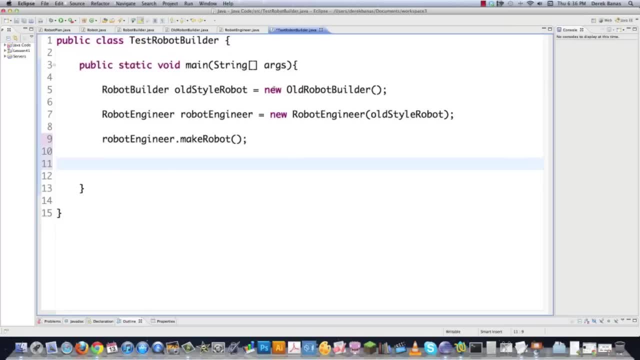 And then the engineer is going to return the right robot based off of the spec that we passed it right here. Now we got ourselves a robot, So we're going to go robot First. robot is what it's going to be called And it's going to be equal to the object that is going to be returned whenever get robot. 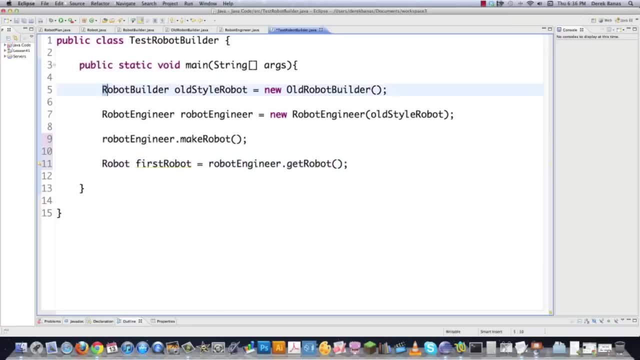 is sent to the engineer. So just to re go over all this stuff: basically we're defining a robot builder right here And this can be thought of as a blueprint for creating a very specific type of robot, And we want a robot to be built for us. 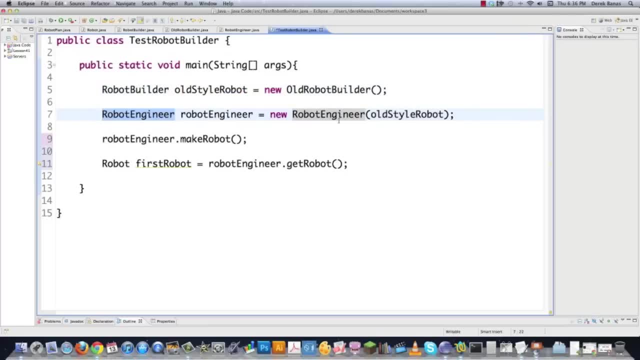 What do we need? We need an engineer to build that robot for us. And to be able to build that robot, the engineer is going to need the blueprint which we defined up here passed over to it. Once it gets the blueprint, the engineer, being smart like he is, can make ourselves. 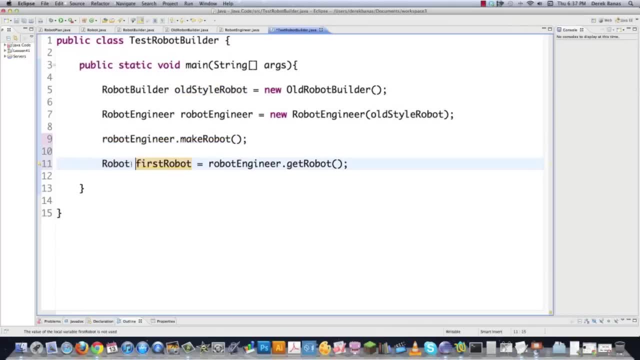 a nice little robot And then we're going to be actually able to define the actual robot and just call robot. get robot from the robot engineer And it's going to pass it over And the robot is ready to go. The robot will be defined and ready for us to work with. 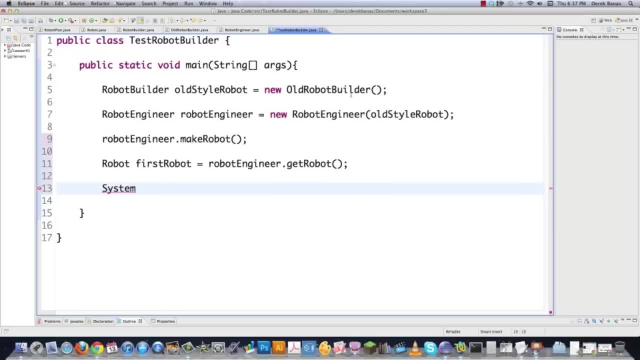 So pretty cool, Especially because nothing knows what's going on, except for this guy up here, the robot builder. So let's check to make sure that we actually did this right And we can say proudly that our robot was built. And then we need to see if our robot was built right. 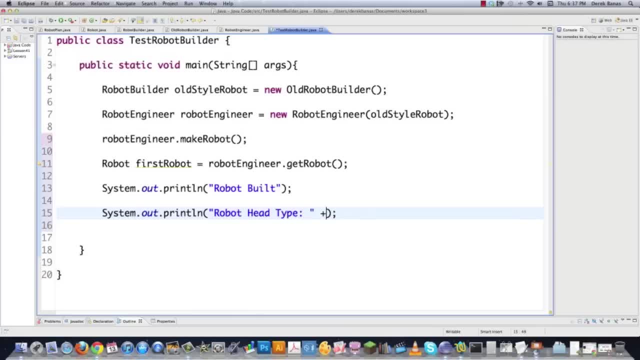 So we can say something like robot head, type like that, And then we just need to go first robot, the object we created, and then say, hey, what is your robot head look like? And it's going to tell us And we can just copy that, paste that inside of there. 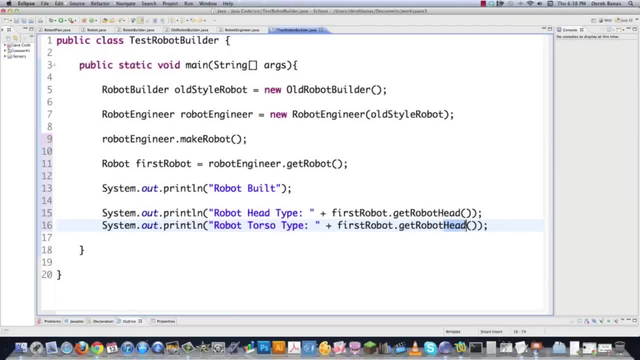 And then we can just change this to: torso- get robot. torso arm type. first, robot get robot arms. If you use nice naming conventions, you don't even have to think. You can just like do this out of your head, which is great. 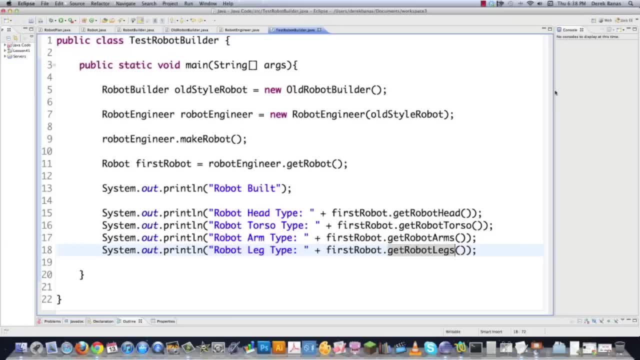 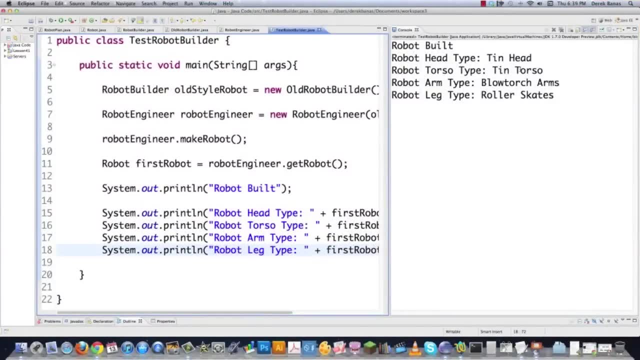 And get robot legs And if we file save that, we can see what type of awesome robot we created there in a very structured manner. And there you go: Robot built Robot head type tin head, tin torso, Blowtorch, Blowtorch arms. 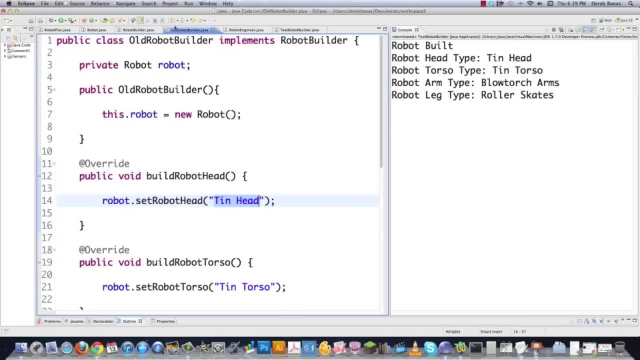 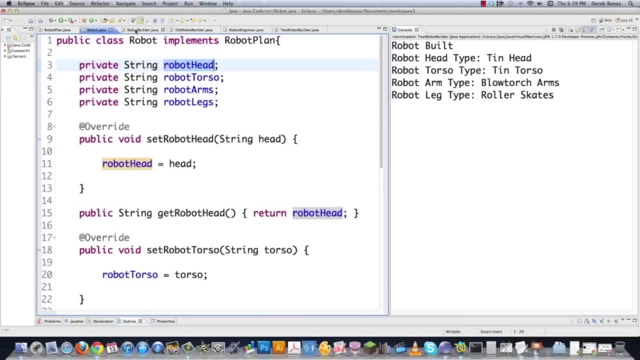 Roller skates Able to put all that together with really only one part of this whole entire builder pattern, Knowing any specifics about the total robots that's going to be created. everybody else is left in the dark and just does their jobs. Leave any questions or comments below. Otherwise until next time. 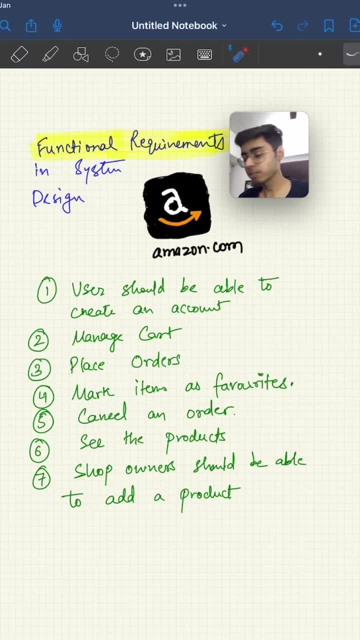 Let's try to understand functional requirements of a system in software engineering, right So whenever you are, let's say, you're building amazoncom, right So the functional requirements of this software or this website or this mobile app should be: user should be able to create an.